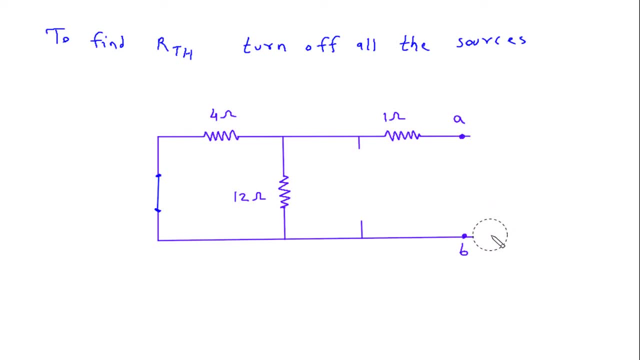 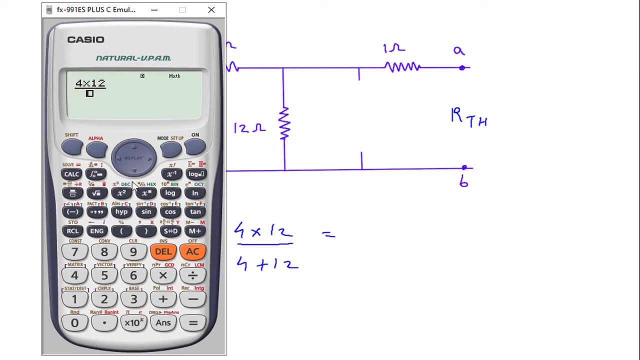 And here, in place of RL, this will be RTH, So this will be 4 Ohm, parallel with 12 Ohm: 4 x 12 x 4 plus 12.. 4 x 12 x 4 plus 12.. 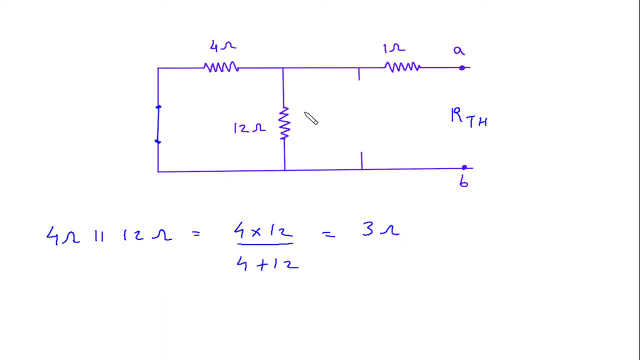 This will be 3. Ohm, So this will be 3 Ohm. Now this 3 Ohm series with 1 Ohm. So 3 Ohm plus 1 Ohm is equal to 4 Ohm. So therefore this total will be 4 Ohm. 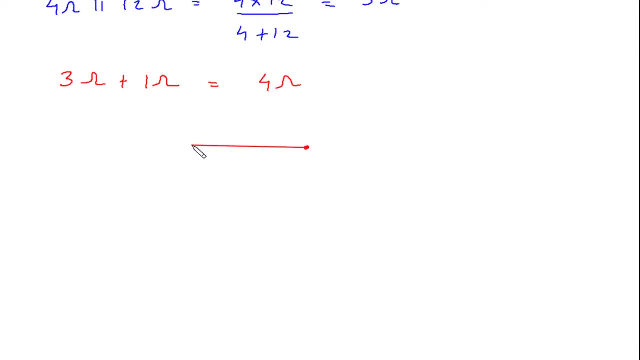 So RTH is 4 Ohm. So RTH is 4 Ohm. So this is- RTH is 4 Ohm. This is terminal A D. This is terminal A, D, A and B. Next we have to find VTH. 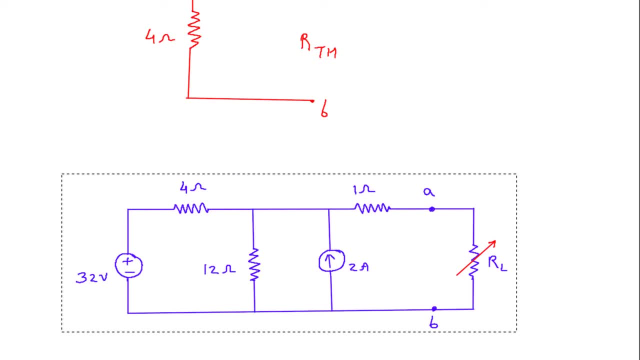 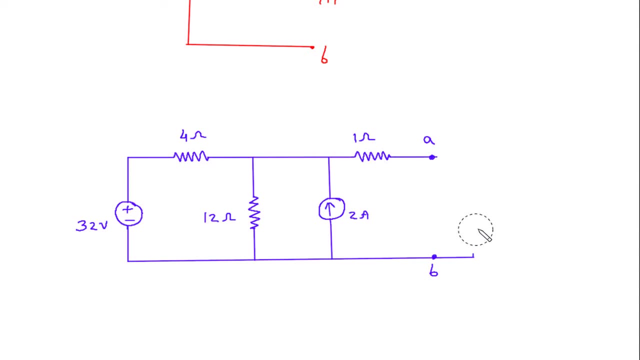 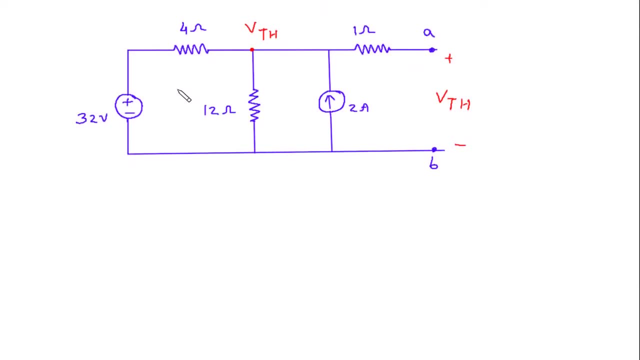 So to find Vth, let's say this is loop number one with current I1,, this is loop number two with current I2, or directly, we will apply nodal analysis. So let's say this is: this is node number A, node A or node number one. 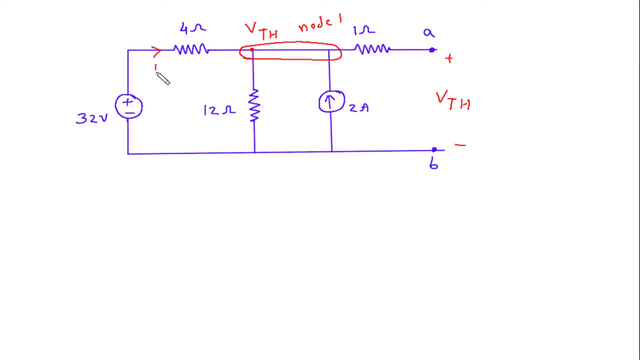 Let's assume the direction of current. let's say this is current I1,, this is current I2 and this is current. this is reference node. This is open circuited, so there will be no current through this resistance. So now apply KCL at node one. 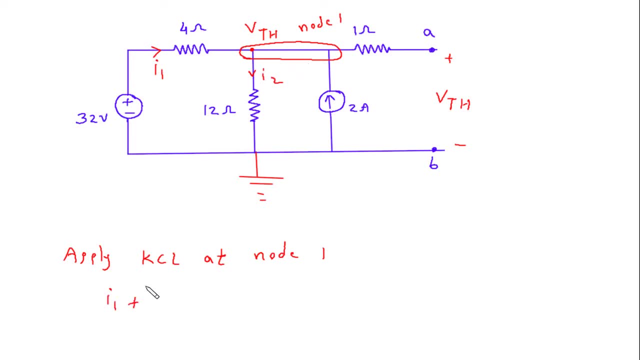 So entering current. entering current is I1 plus 2 ampere. summation of all the entering current is equal to leaving current. leaving current is I2.. So this will be I1 will be 32 minus Vth, 32 minus Vth by 2 ampere. 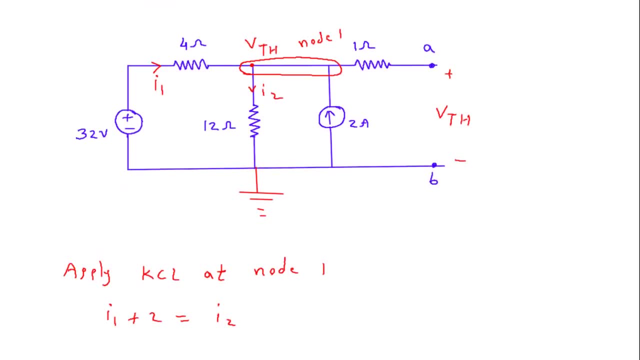 So this will be 32 by 4. ohm plus 2 is equal to I2.. Now this I2 is Vth minus 0 by 12, Vth minus 0 by 12.. So this will be 32 by 4 minus Vth by 4.. 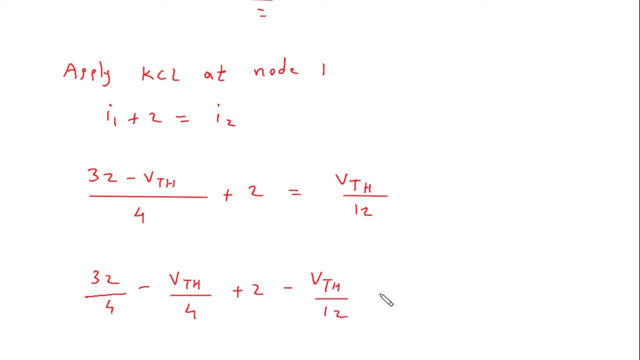 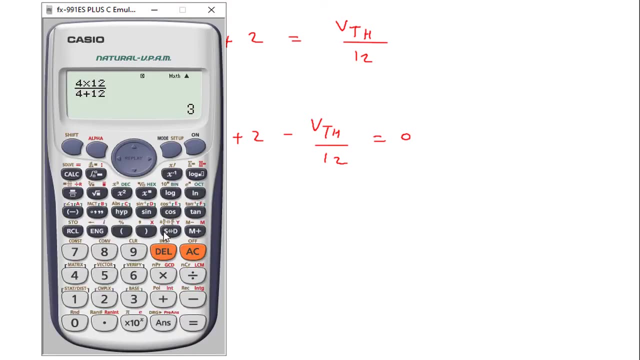 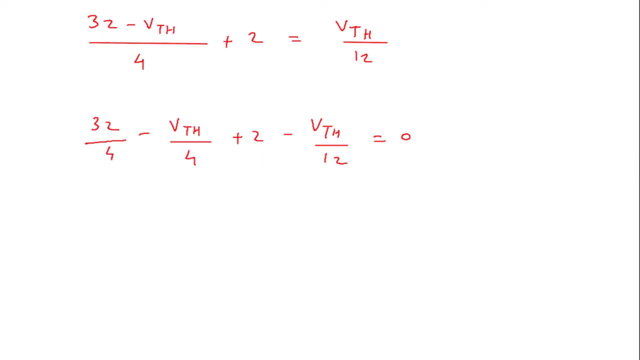 Plus 2 minus Vth by 12 is equal to 0. So this will be 32 by 4 plus 2.. So this is 10 and this will be minus 1 by 4.. Minus 1 by 4.. 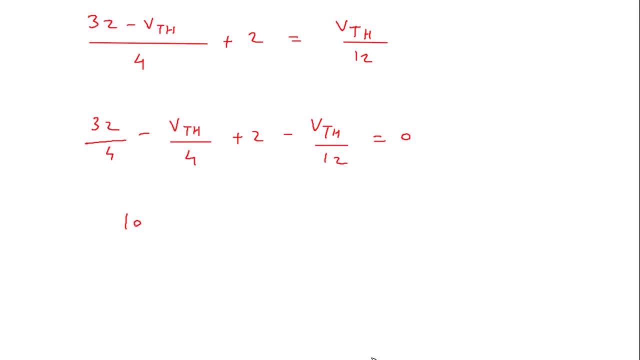 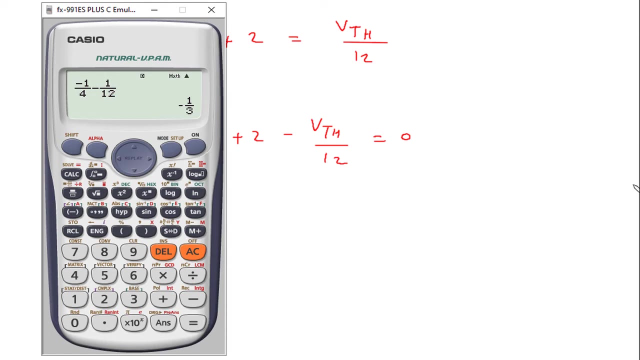 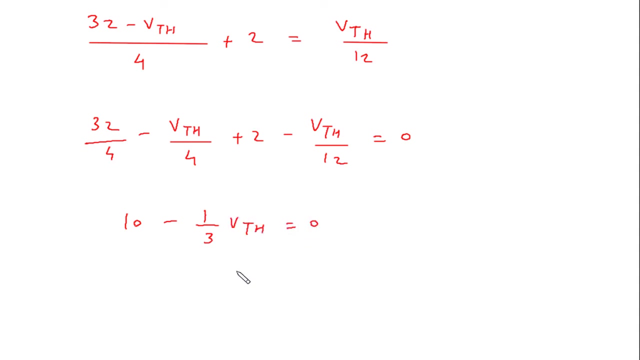 Then minus 1 by 12. Minus 1 by 12. So minus 1 by 3, minus 1 by 3, Vth is equal to 0. So this will be: 1 by 3. Vth is equal to 10.. 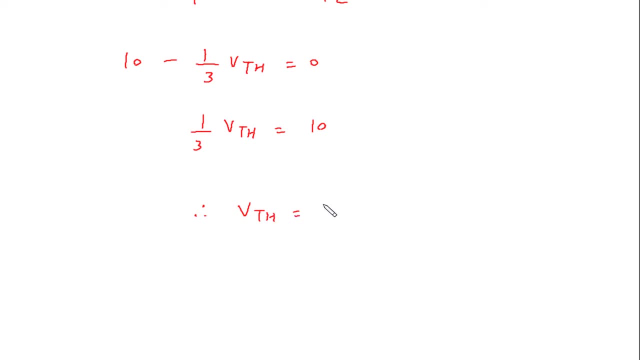 So therefore Vth is equal to 30 volt, So Vth is equal to 30 volts, 30 volt and Rth is equal to. Rth is equal to 4 ohm. Now we will draw the thevenin equivalent circuit, So thevenin equivalent circuit will look. 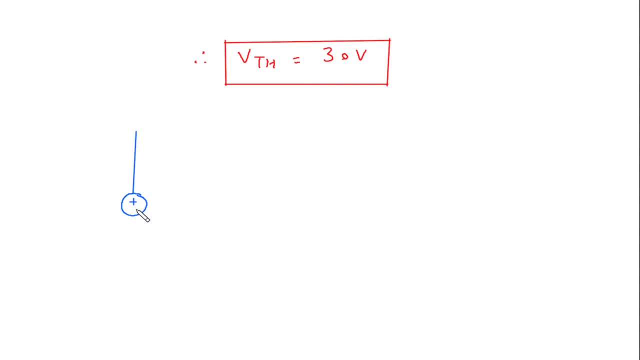 like this. This will be positive. negative. This will be. this is Rth. This is Vth. Vth is equal to: or. here we will write: Vth is equal to 30 volt. Rth is equal to 4 ohm. 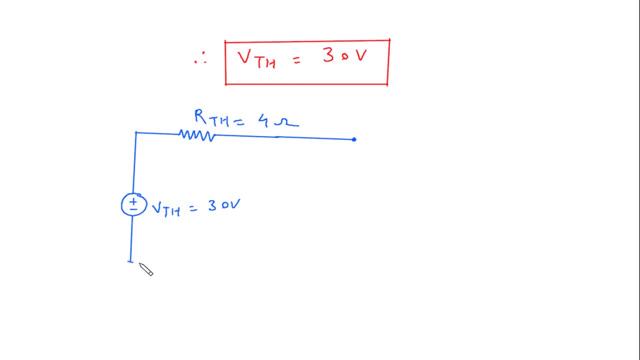 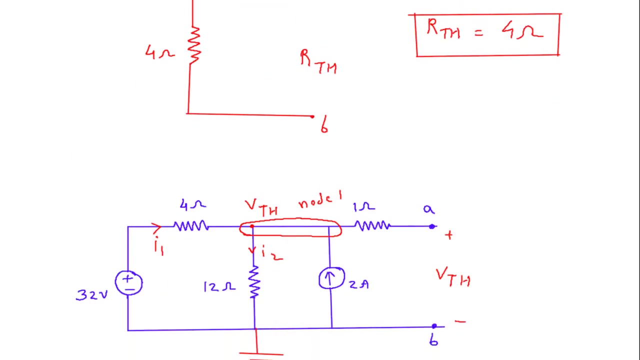 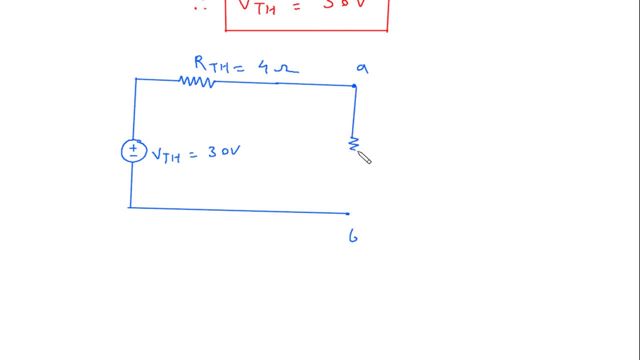 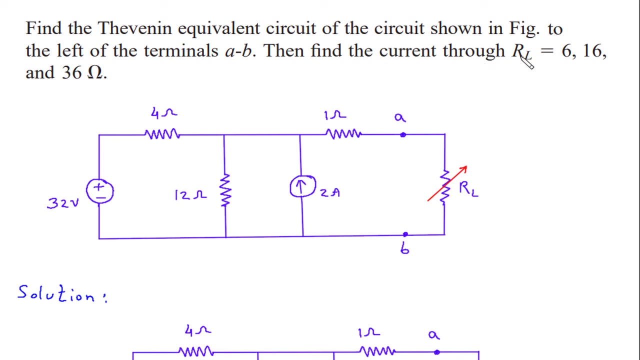 And this is terminal Terminal A and terminal B, And in between terminal A and B, RL, which is variable register or load register. This is RL. Now what we have to find. We have to find, then find the current through RL. So RL, we 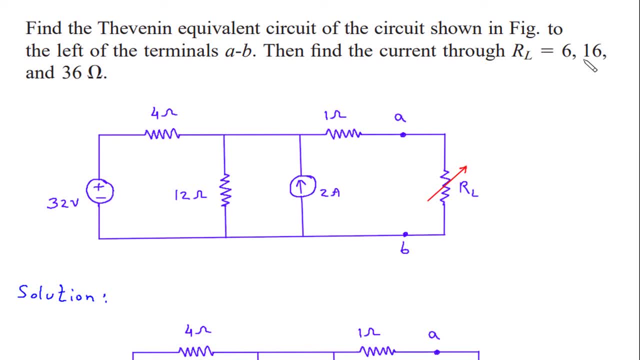 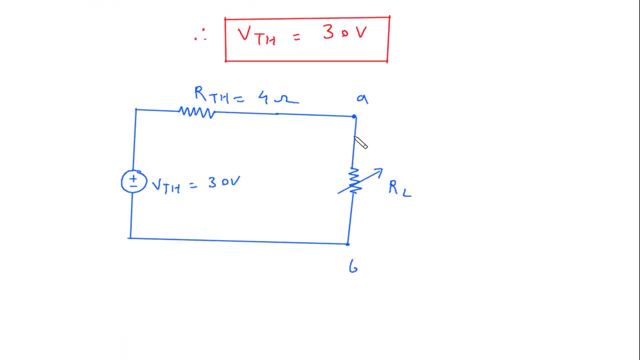 have to find IL When RL is equal to 6.. 16 and 36. So we have to find this IL. So IL is equal to Vth, Vth, Vth By Rth plus RL, Now when RL is equal to 6. When RL is equal to 6, then 6 ohm, then IL is. 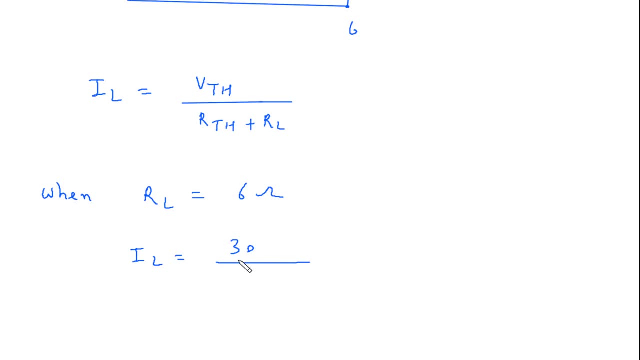 equal to Vth, which is 30.. By Rth, which is 4.. So for of the control, the strength of RL, because RL plus 13 is equal to 30, by which is 4.. So 4 plus RL is 6.. So this will be 10.. This will be 3A. Now, when RL is equal to 16, then 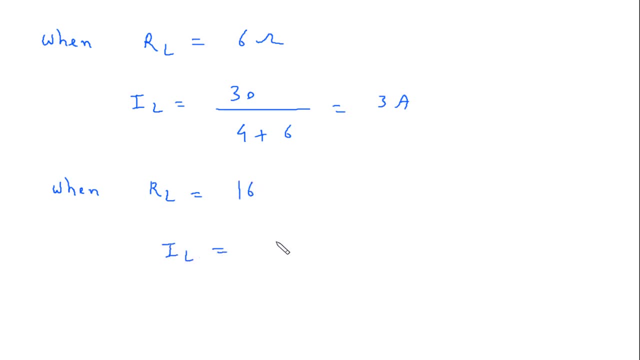 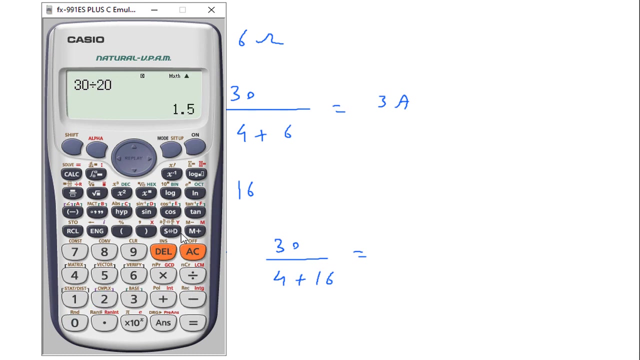 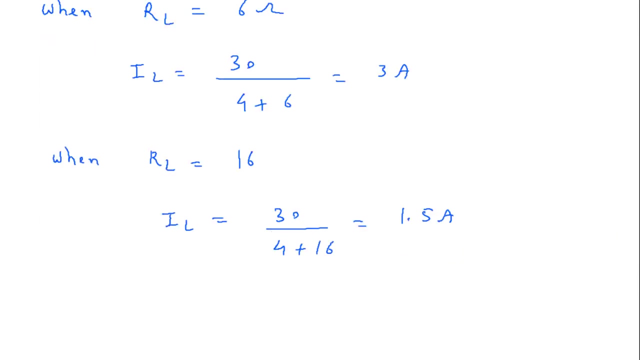 IL is equal to 30 by 4 plus 16.. So get something between R and 14, which will be 6.. So the difference will be what Bs insight, 4 plus 16. so this will be 30 by 20, 30 by 20, which is 1.5, 1.5 ampere. then, when RL is equal,